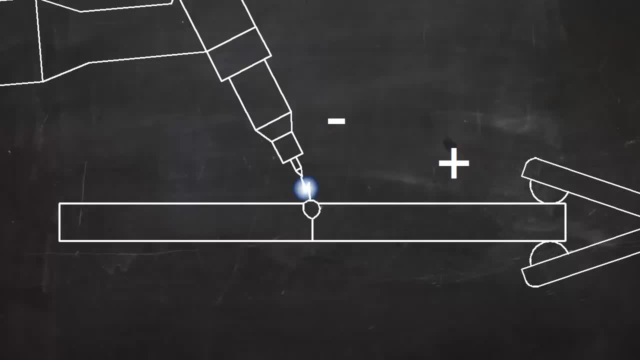 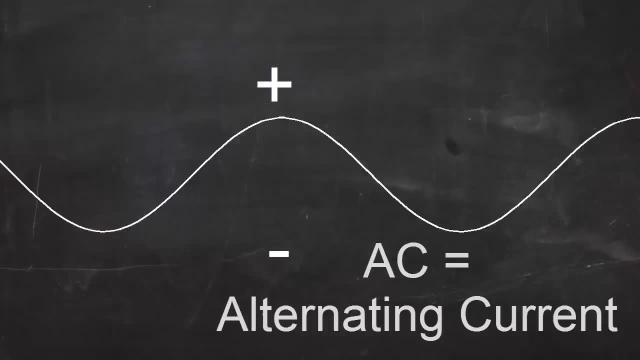 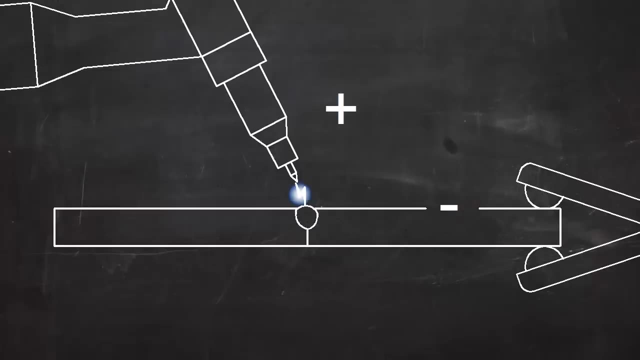 descriptive term. DCEN puts most of the heat on the workpiece and it's the most common setup When welding aluminum, however, AC is used. In AC, the positive and negative voltages switch back and forth between the electrode and the workpiece. This puts more heat on the electrode, but 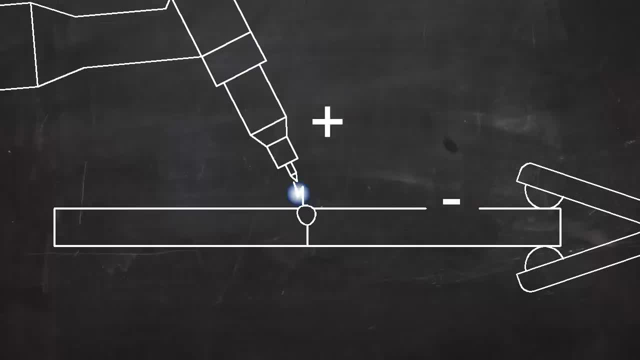 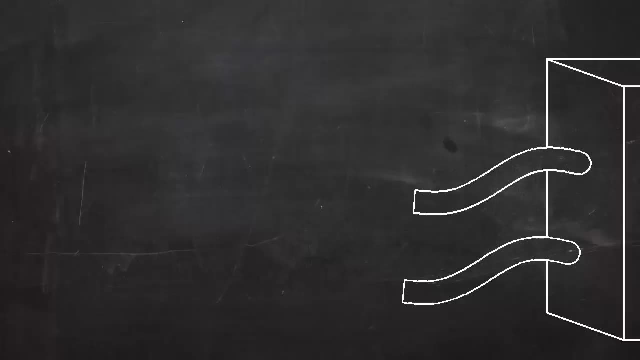 it has a cleaning effect on the workpiece. You see, aluminum forms oxides that float to the top of the weld pool and prevent a good weld. AC current helps control these oxides. AC current helps control these oxides. In an electric circuit the current flows in a loop. In TIG welding the current has to flow. 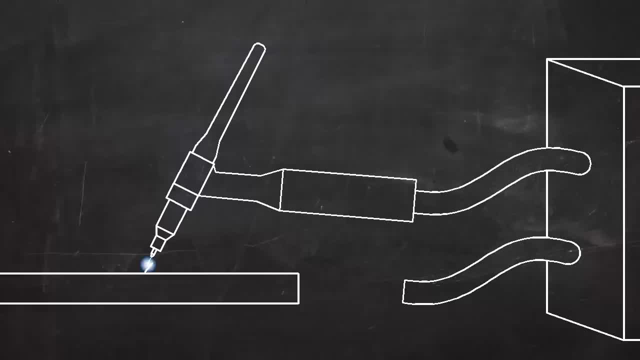 in a complete circle from the machine to the torch, into the work and back to the machine. A work lead is clamped to the work to complete the circuit from the workpiece back to the machine. Now you can TIG weld with or without filler metal and that's not a choice you have in a lot. 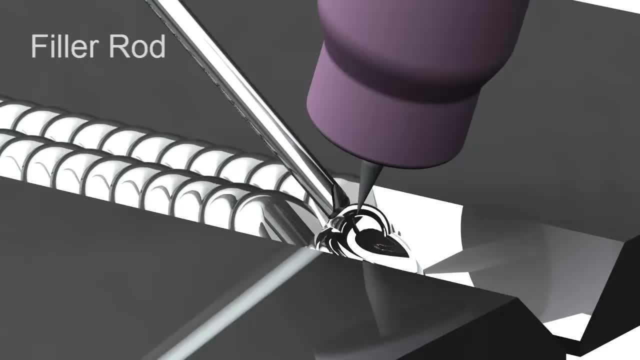 of other processes. If you want to add filler metal to a TIG weld, use a filler rod, which is just a rod of metal with a specific output. You want to make sure that the filler metal you're using is compatible with the base metal. 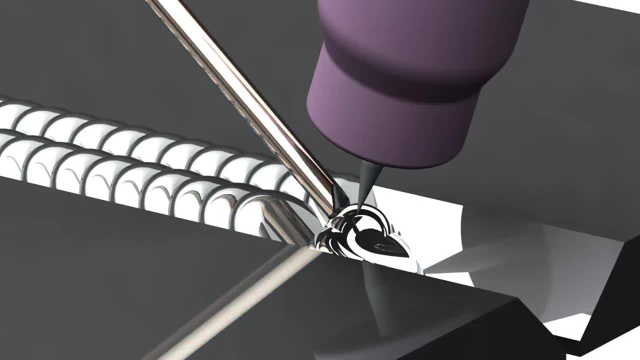 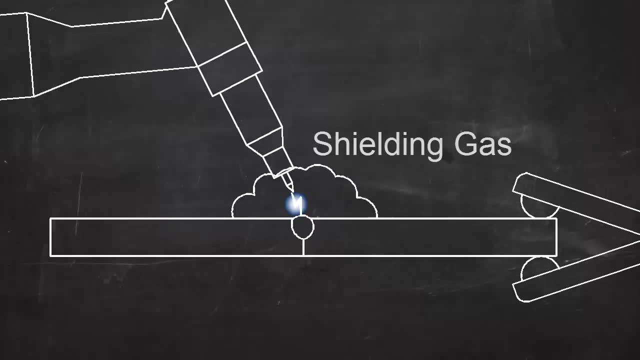 and that it has the strength required to do the job. In TIG welding, the molten metal is protected by a shielding gas. This gas- usually argon and sometimes helium or other gases- keeps the molten metal from reacting with oxygen. 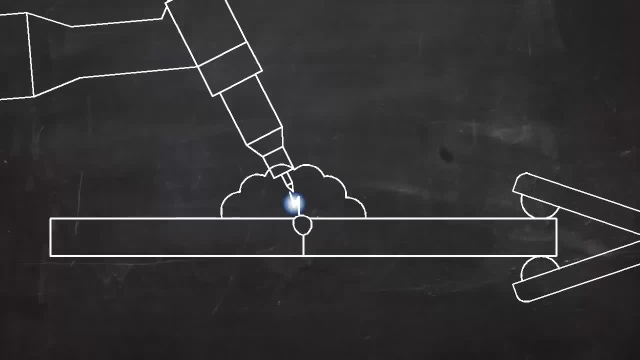 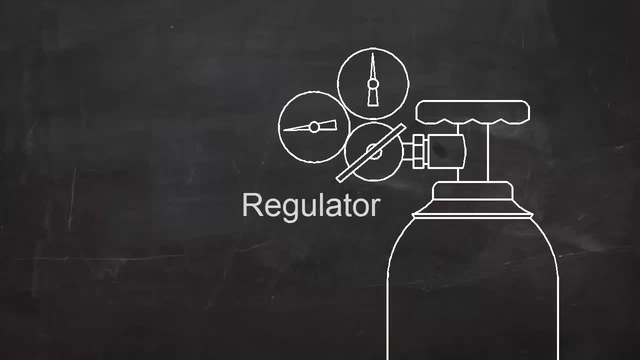 water vapor and the atmosphere. This shielding gas is stored in high pressure cylinders like these. The pressure is reduced to a usable level by a device called the TIG weld a regulator. The shielding gas flows through a hose and comes out right at the point of the weld. 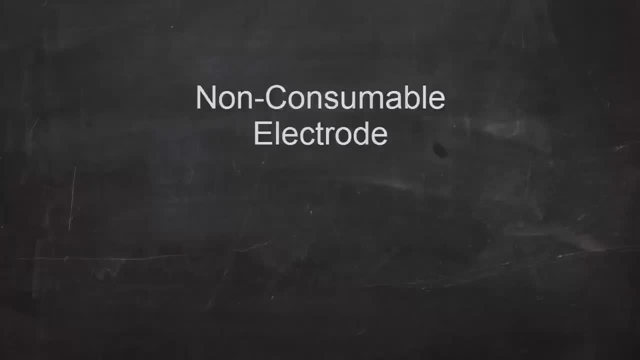 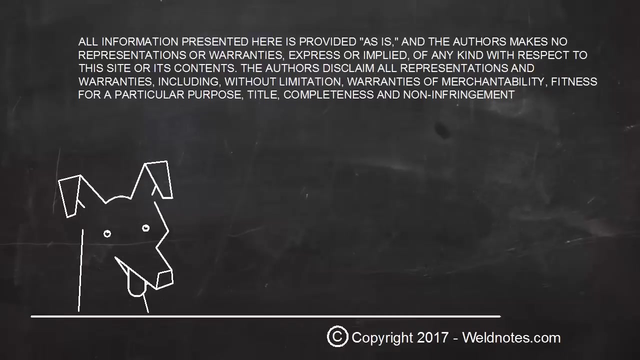 So, in summary, TIG welding is an electric arc welding process, uses a non-consumable tungsten electrode, the filler metal is added separately in the form of filler rod and the shielding gas comes from a high pressure cylinder. Thank you for watching.